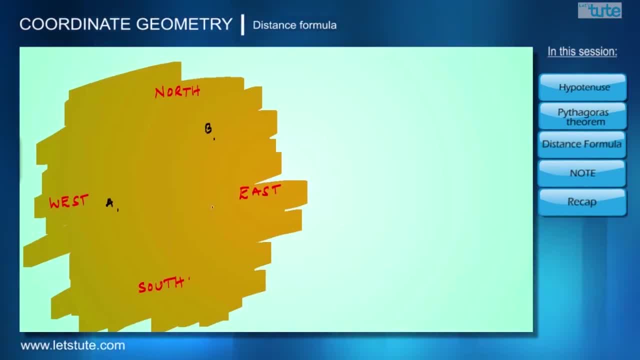 to go to town B but they have to travel via town C. Town C is over here and this town C is at 4 kilometers in the east direction of town A and 3 kilometers in the south direction of town B. That means if anybody wants to go to town B from town A via town C, they have 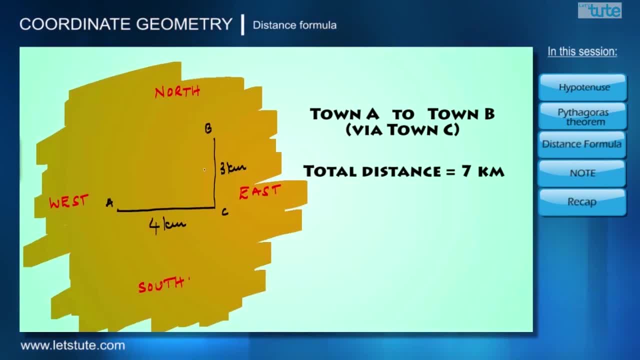 to travel total of 7 kilometers. So they thought of preparing a way directly from town A to town B, which may take less time to reach town B and people may have to travel less distance. But what is the direct distance from A to B? If you notice this, it is forming. 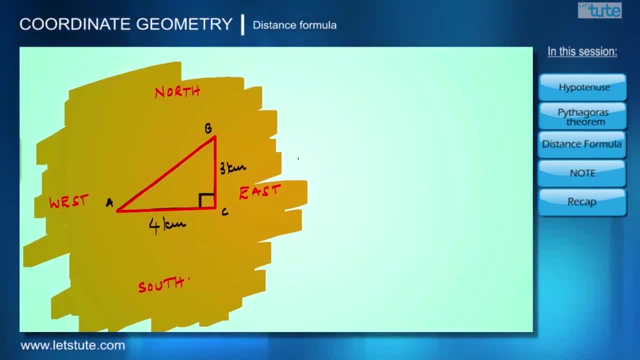 a right-angled triangle with right angle at C and side opposite to right angle is called as Hypotenuse. that is nothing but, in our case, distance between A and B, And we can find this length of Hypotenuse using Pythagoras theorem, and we already know that Pythagoras. 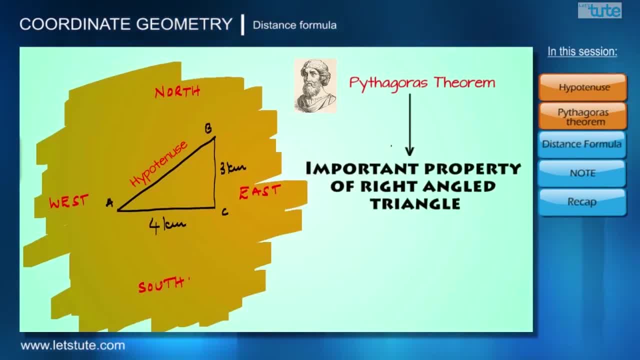 theorem is one of the important property of right-angled triangle angle and it is useful in finding the length of the hypotenuse. It states that square of the length of the hypotenuse is equals to sum of the squares of the remaining two sides. 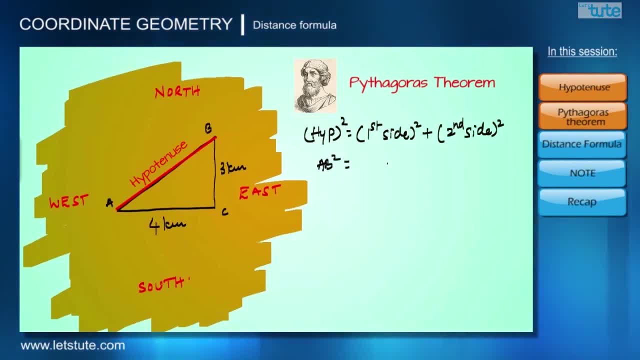 So in our case hypotenuse is AB and remaining two sides are AC and BC. So this can be written as: AB equals to square root of AC square plus BC square. We know the values for AC and BC, so on putting those values we get AB as 5 kilometers. Here we see that for finding distance. 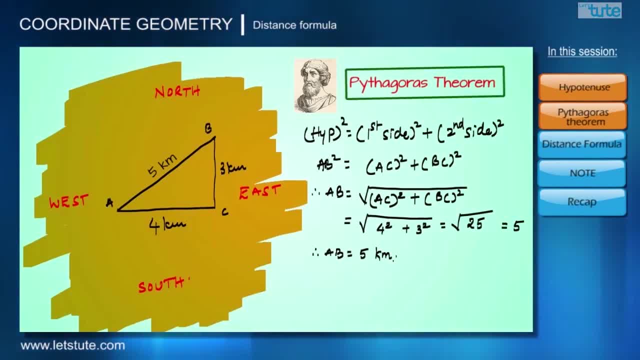 between two towns. we use Pythagoras theorem because we were knowing absolute distances. What if, instead of absolute distances, we are given with coordinates of those two towns? So let's say A is X1- Y1 and let's say B is X2- Y2.. Now A is X1 units away from the origin. 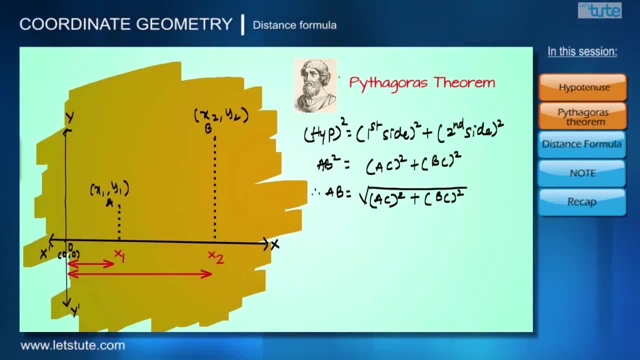 and B is X2 units away from the origin on the X axis. Now we can find the length between X1 and X2 by subtracting this small length X1 from this big length X2.. So therefore, length between X1 and X2 becomes X2 minus X1.. Similarly, A is Y1 units away from the origin and B is 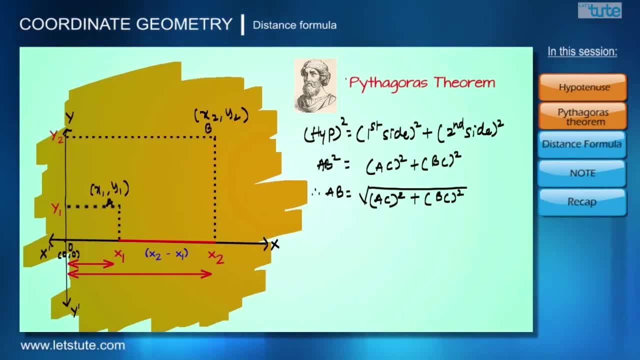 Y2 units away from the origin on the Y axis. Therefore, length between Y1 and Y2 will become Y2 minus Y1.. And now we want distance between A and B. Let's draw AC perpendicular so that it forms a right angle triangle, ABC, with right angle at C and side opposite to right angle is AB. 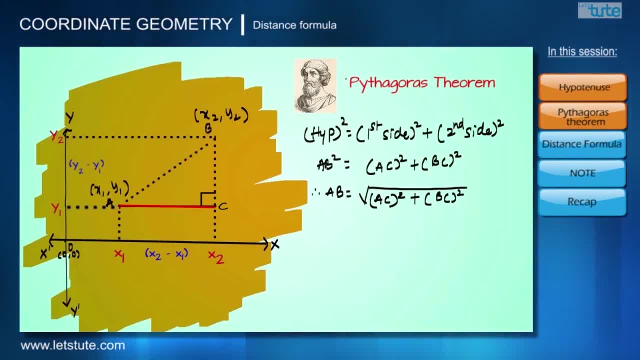 Now, AC is parallel to X1, X2 and it is equal in length. Therefore, AC will also become X2 minus X1.. Similarly, BC is parallel to Y1- Y2. it is equals to the length of y1, y2.. So therefore, bc will become y2-y1.. And, as we know, for finding 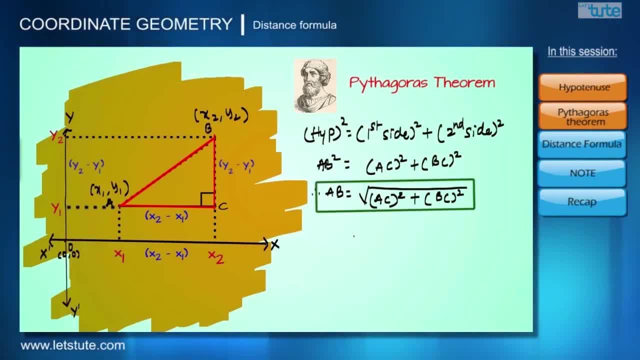 the length of the hypotenuse. we use Pythagoras theorem, which we already have here. So by putting the values of ac and bc in Pythagoras theorem we get ab equals to square root of x2-x1, the whole square, plus y2-y1, the whole square. Now this is called the distance formula. 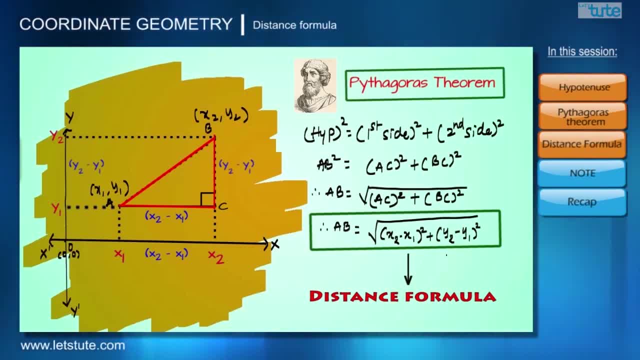 And we have derived this using Pythagoras theorem. If you know the values of x1-y1 and x2-y2, we can apply them in this distance formula for finding the length between the two points. So let's see how it works. So let's take coordinates for a as 3,2 and coordinates for 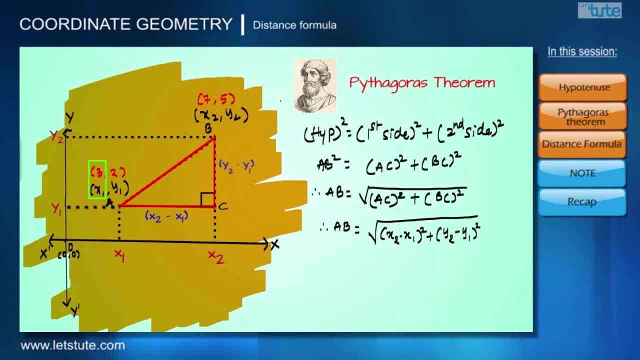 b as 7,5.. So now we can see that x1 is 3, y1 is 2, x2 is 7 and y2 is 5.. So therefore, when we use distance formula for this, we get ab equals to. 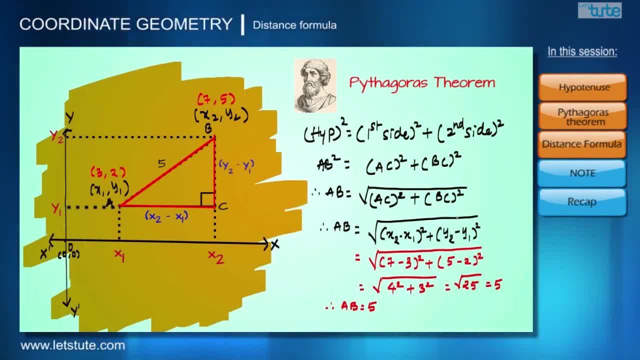 5. And if we know the absolute distances of ac and bc, ac is nothing but x2-x1, which will be 7-3, 4, and bc is nothing but y2-y1, which is 5-2. that is 3.. On using Pythagoras theorem: 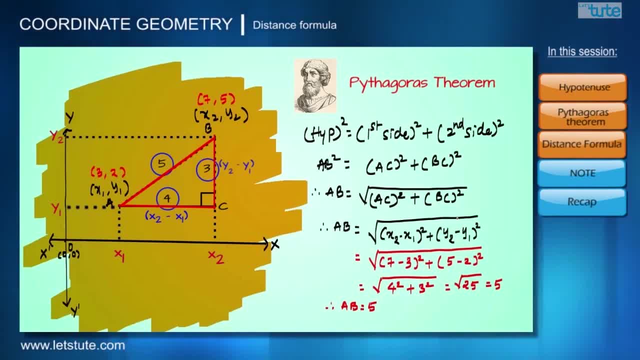 on the absolute distances 4 and 3, we get hypotenuse as 5, the same distance. So what do we understand from all this? That distance formula is derived from Pythagoras theorem And both useful in finding the distances. The only difference is Pythagoras theorem.